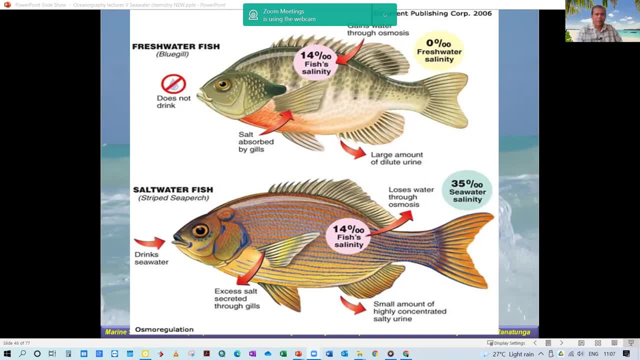 another. that's mainly because of the amount of water, that's this chemicals being dissolved. that's mainly because of the amount of water that's this chemicals being dissolved is a different, and that's where we have different salinities in different environments Right now. 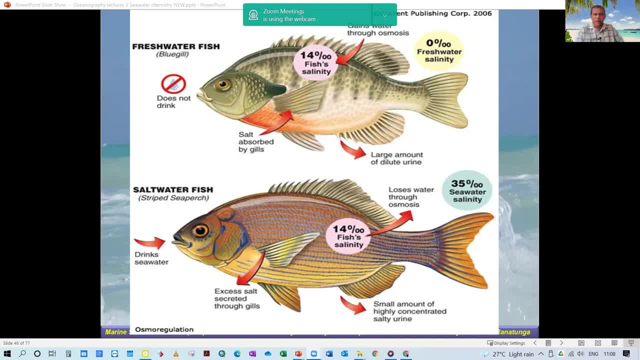 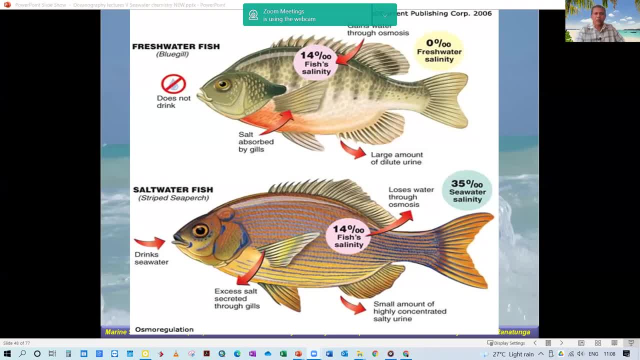 salinity in different environments would cause a lot of issues in the marine organism, not only the marine, even the freshwater. So for the aquatic organisms the amount of dissolved substances is going to play a key role. Last week we discussed that: the freshwater and the saltwater- it's very different. 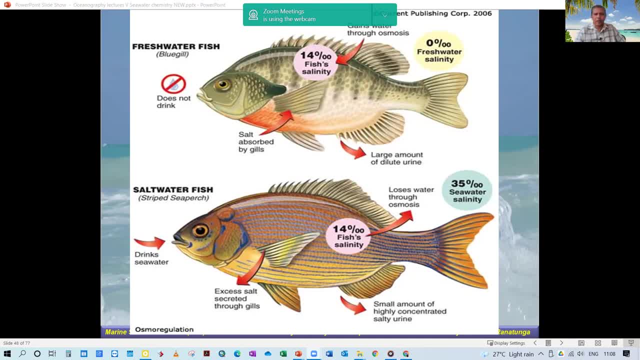 And the effect on the animals or the aquatic organisms is different. For example, in the freshwater the animals tend to get water inside their body Because the water concentration outside is high and inside the body is low. you know, the water always try to go from the high concentration to the low concentration. 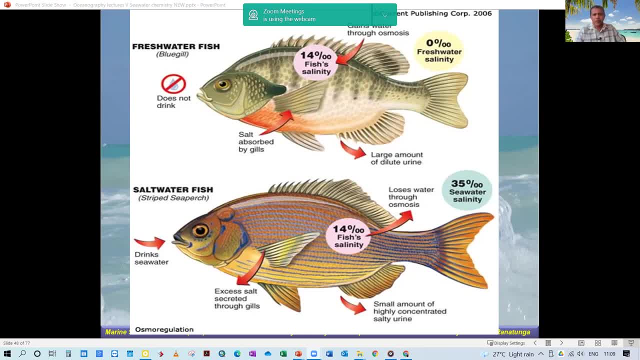 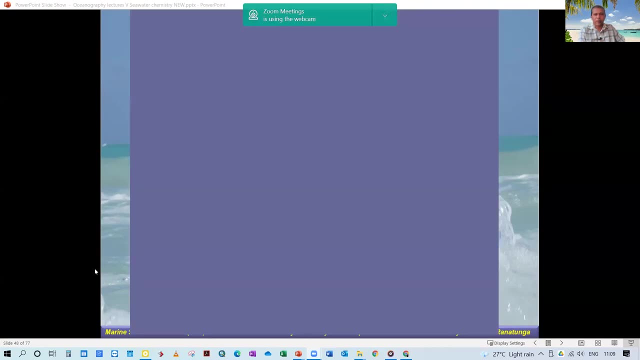 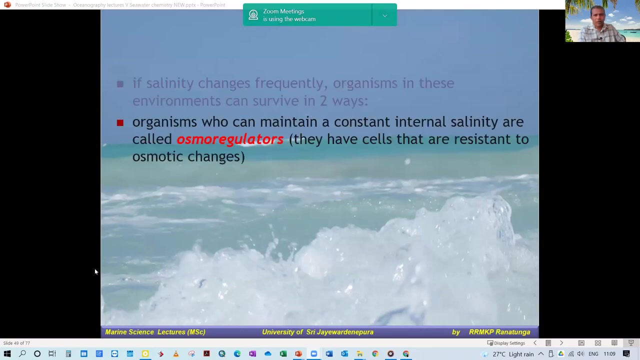 But on the other hand, the marine organisms: they lose water because the outside concentration, the water concentration is low, So they have to deal with this phenomenon. So we actually learn these things in the Ecology. I mean these are ecological aspects in the marine organism. 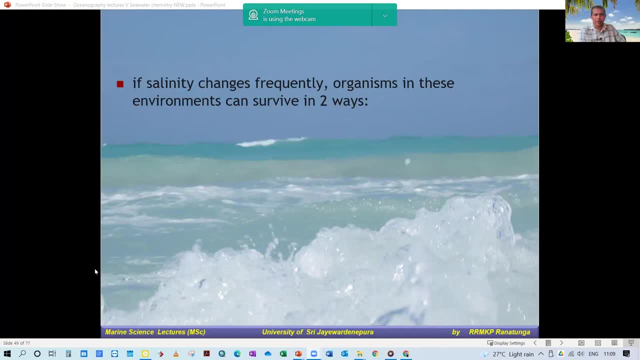 So the animals have some adaptations, or they should have some adaptation to cope with these changes. So that's how some organisms, some marine organisms, they are called the osmoregulators. So no matter what is the salinity outside, they maintain their internal salinity. 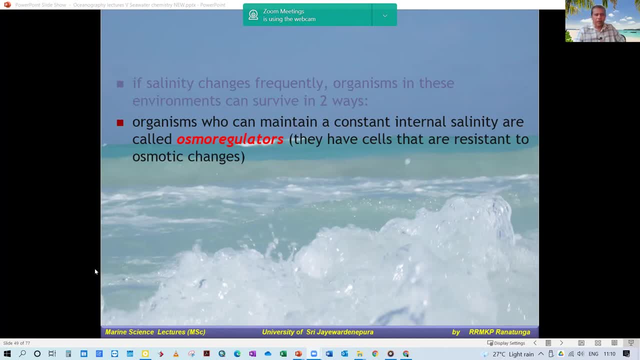 So the internal salinity or internal constituents in their body fluid. I have done a lot of research on the body fluid. We call the osmoregulators for them, While the others are osmoconformers, where they have to change their internal body salinity or the dissolved salt. 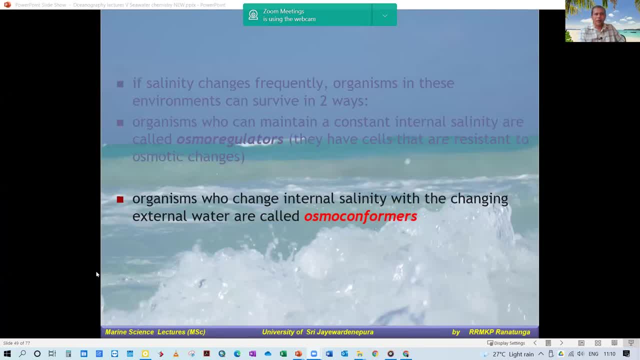 With the changes in the environment. The osmoconformers, The same with the thermoregulators and thermoconformers. Some animals can regulate their temperature, Whereas the other animals like reptiles, a lot of invertebrates. 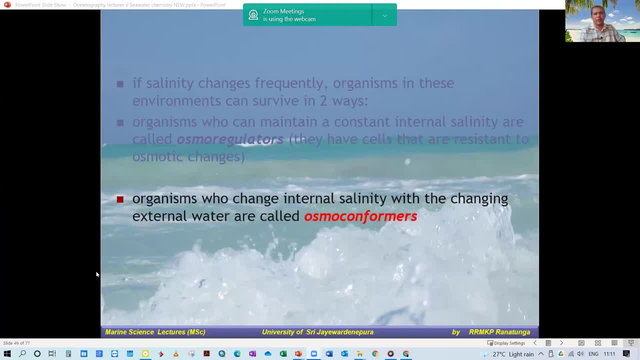 they have to change their internal body temperature with the change in environment. Similarly, the aquatic organisms has to deal with the salinity changes, either becoming osmoregulators or conformers. But even with that, there are other organisms also who can tolerate the salinity changes. 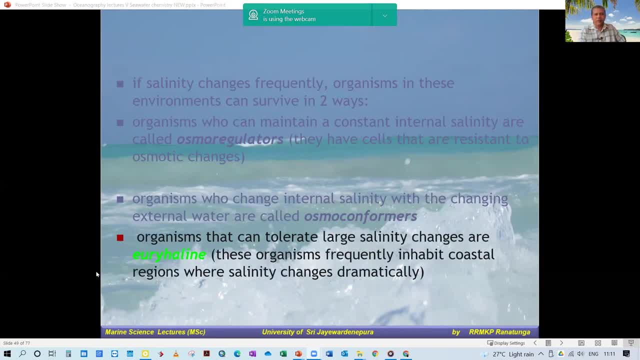 We call them as the urehaline organisms. Like a species living in the coastal zone, especially in the lagoons, they might be urehaline. They have to deal with zero salinity. sometimes, During the rainy season, fresh water will bring the salinity down to zero. 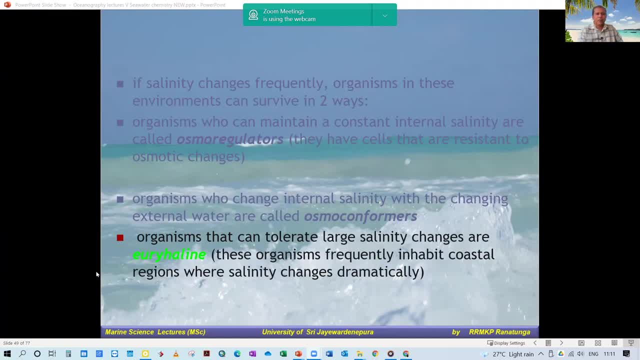 But sometimes it will be 5,, 10,, 20.. Sometimes, even with the tide, even the salinity can go up to 30, something like that. So they have to adapt to that salinity changes, So they have to have some adaptation. 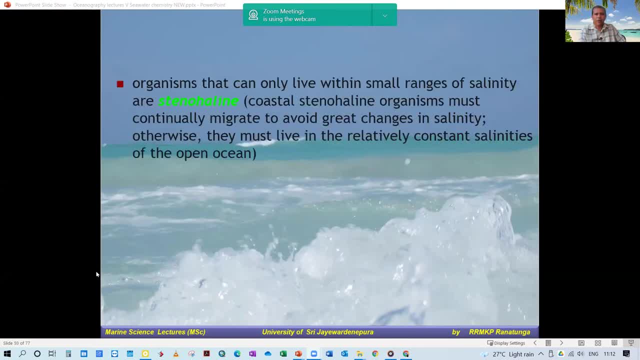 These are some of the issues that the marine organisms have to face, Whereas the other organisms- some- are very sensitive to salinity changes, So they have to avoid salinity changes, Like if they are living in the coastal zone, if the salinity changes. 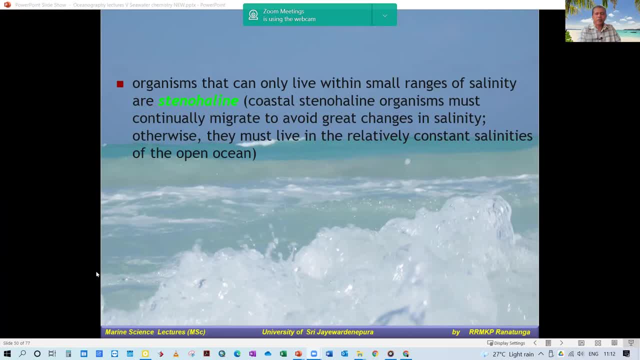 they have to move here and there. So that's why some fish, some prawns, some organisms, they migrate from one place to another to cope with the salinity changes. So you see now this chemistry, how it's affecting the animals. 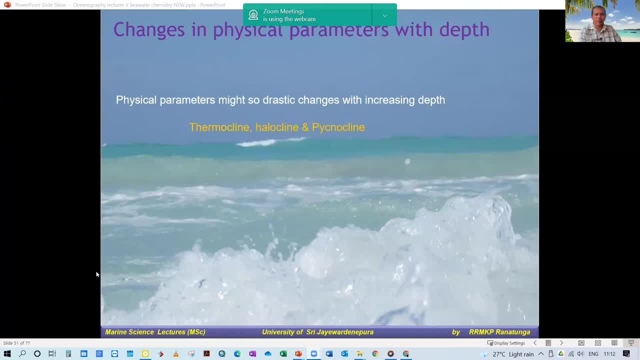 So there are a lot of things associated with these things. As I mentioned, we can't talk a lot, especially with the. We are putting a lot of things into the seawater And the ocean chemistry is being changing, which is going to cause a lot of issues. 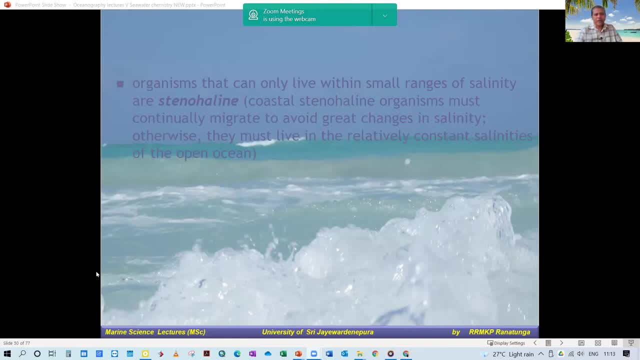 like what we talk about: the climate change. Of course, global warming, as well as the reason for climate change, especially the ocean acidity. But we will talk these things towards the end when we discuss about the issues in the marine environment. But keep in mind 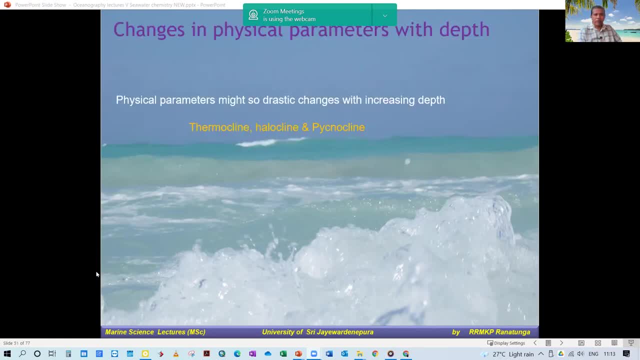 that we are changing the ocean chemistry, which eventually will have other consequences soon. So now we'll very briefly look at how these chemical constituents, or any substances that dissolve in seawater, how they change with the depths, Especially in the ocean. we have to talk about these depths. 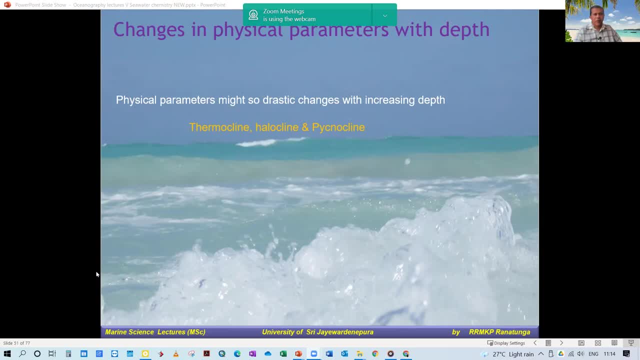 because from the coastal zone where the depth is not that high, it can go up to very high depths. So these some of the physical parameters. they change with the depth, So how it's going to change especially, there can be some drastic changes. 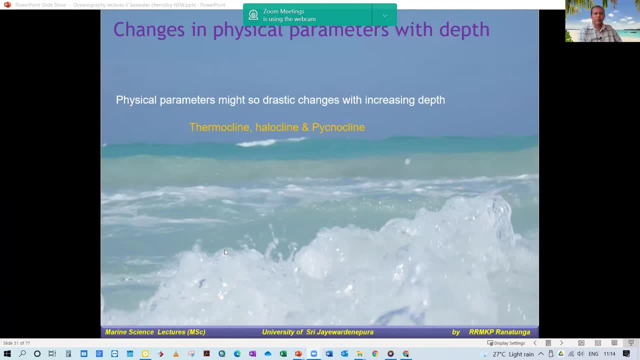 in some of the physical parameters. For example, the temperature may be high in the top layers, but sometimes the temperature can be very low in the bottom, And in between there is a huge change in the temperature, which we call this, the drastic change. 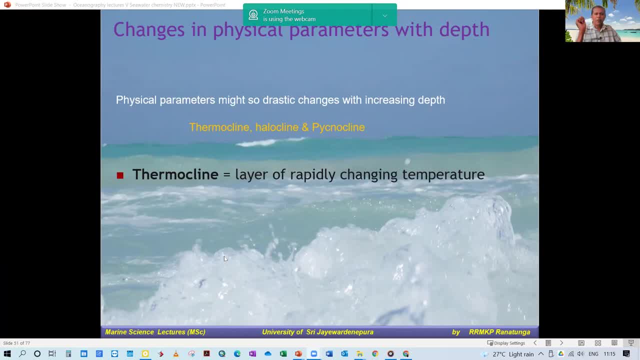 we call as the thermocline. I don't think you have heard this term- Perhaps for limnology you might have discussed this term thermocline- But it's a very important phenomenon in the water, especially in the deep waters. 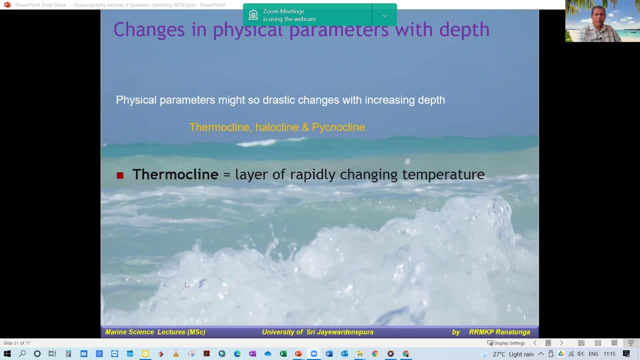 Thermocline, a layer of rapidly changing temperature, And similarly there is halocline, where the salinity changes drastically or rapidly within the short distance, but in a huge difference in the salinity. And similarly there can be a pycnocline. 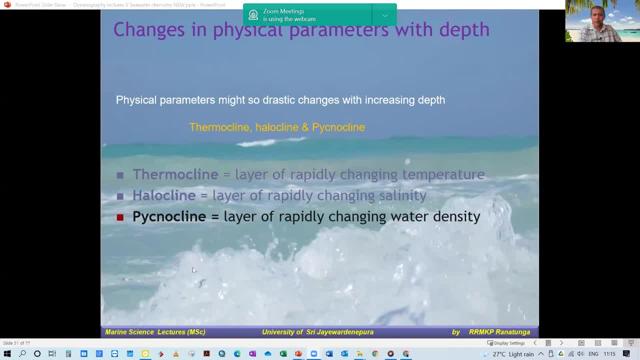 where the density is also different from place to another. I mean sudden or rapid change in the in these physical parameters. Now, these changes, we can, these clines, whatever the thermocline, halocline, pycnocline. 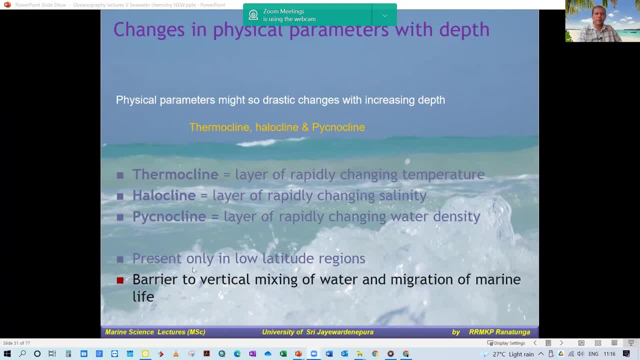 they are very important, especially the. they are also a barrier for the, the, the animals living in the this environment, because if the temperature is very high in the top but very low in the bottom, the bottom water species won't be able to go to the surface. 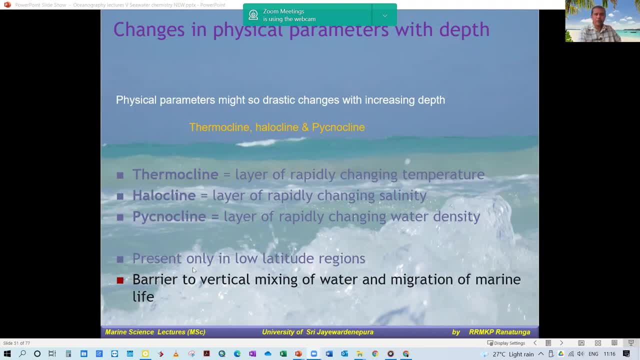 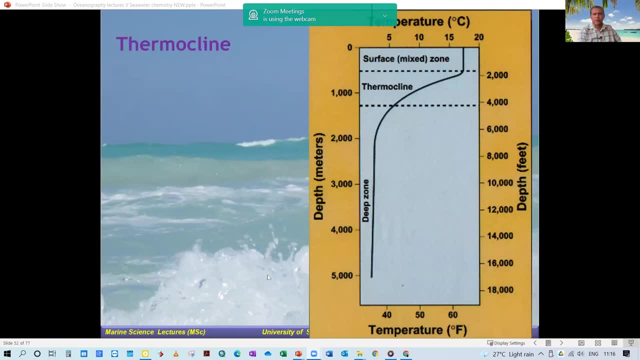 and surface water species won't be able to go to the bottom because it's huge difference in temperature. Similarly, the salinity as well, right? So if you put this one in a graph, this is how it would look like, right. 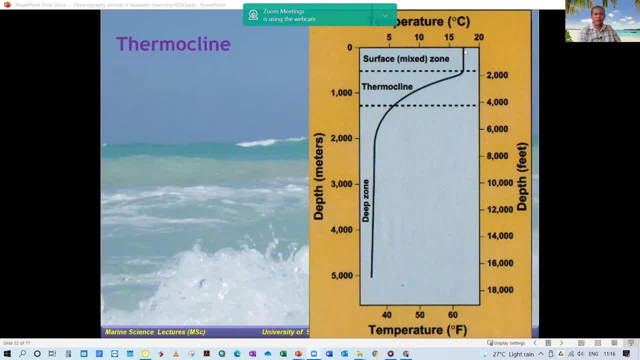 This is the. if you measure the temperature from the surface to the bottom, like here, up to 5000 meters, so five kilometers, you see the change in temperature. see, In the top layer we call the surface layer or the mixed layer. 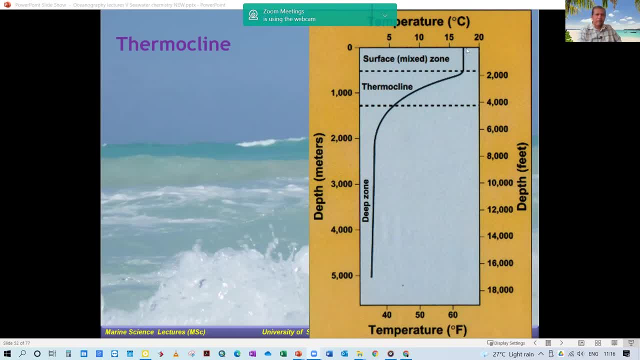 well mixed layer. the temperature difference is nearly invisible, like there's no huge difference in the temperature Here, but you see the bottom temperature, that in the deep waters the temperature is very low but you can go in even up to zero sometimes. 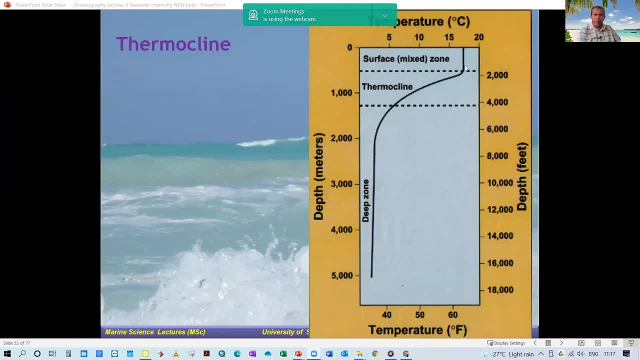 but virtually it's not. But in between, you see, there's a huge difference in temperature and this is the zone where we call as the thermocline single-link kinematics. So because the surface layers will mix, because of the 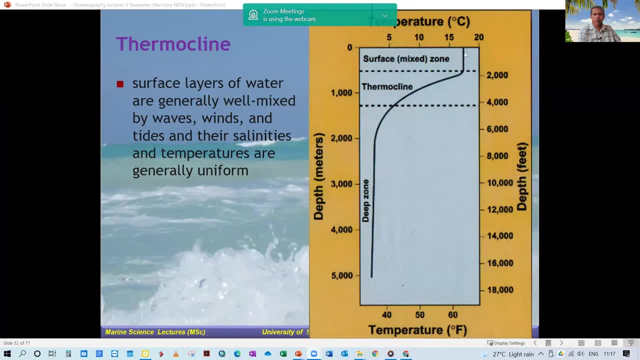 the waves and wind action, well mixed, so temperature is constant. but in the bottom waters not getting enough sun rays and there's no heat generation, so the temperature is very low and in between you have this thermocline. and in the tropical waters you see the the surface layer, mix layer. 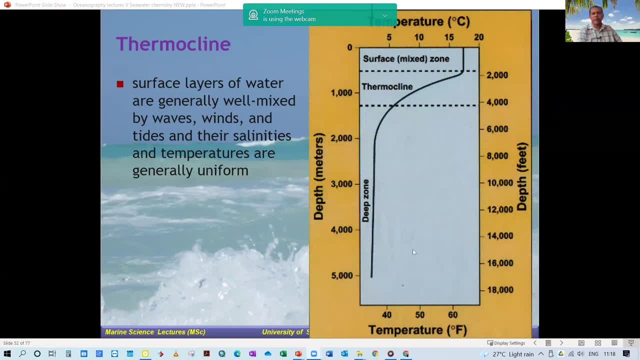 and the bottom layers. there is no chance of mixing. because the bottom waters are cold, the surface waters are warmer. we know that warm waters are less denser, whereas the the, the cold waters are denser. right, density is high here, density is lower here and because of that, 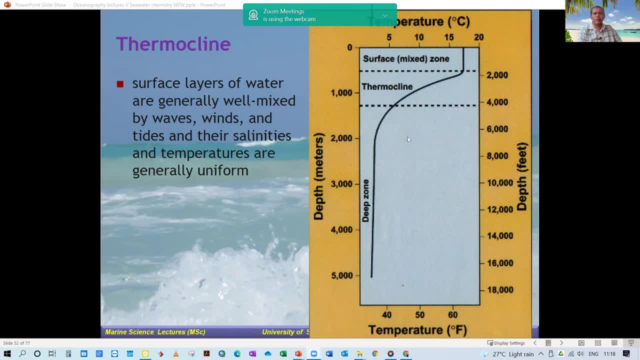 this water going to be remain here as bottom waters and the surface wall will be remain as surface waters and there is no mixing in between the surface and bottom waters. so this is extremely bad for the marine environment. why? because we know the nutrients. usually they are heavier, they sink to the bottom because the because 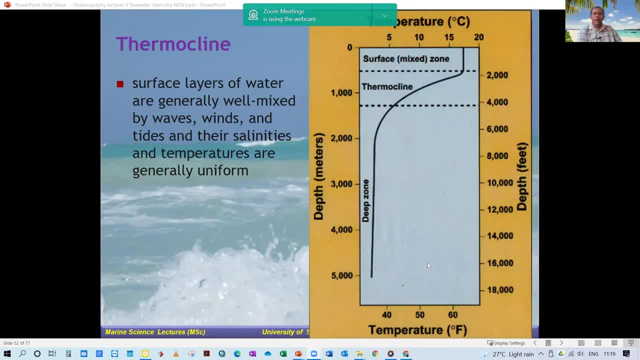 of their heavier, they sink to the bottom and the all the nutrients, will be in the bottom, whereas the, the, the oxygen, will be mostly in the surface, whereas these oxygen has no much chance to go into the deep water. you see, this is bad for the animals because they don't have- especially the animals living in the boat- deep waters. 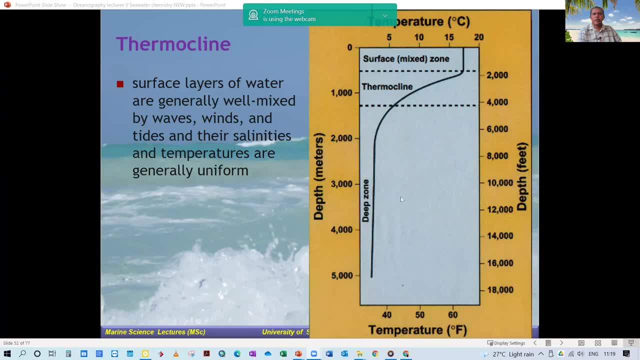 they don't get enough oxygen, whereas in the nutrients point of view, the surface layers were the most productive. the planktons and algae are there. they need the nutrients too for the primary production. so they don't get enough nutrients for this primary production production. so you can imagine the tropical waters in particular. there is no good mixing. 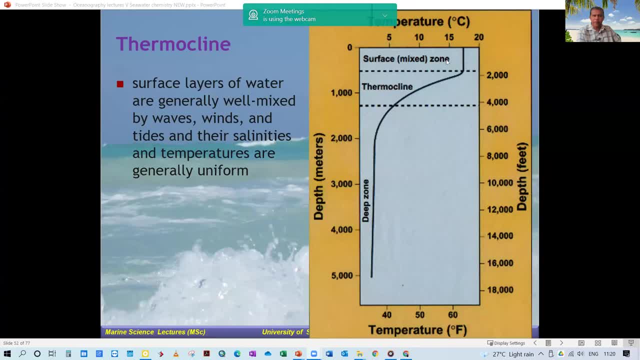 and because of that, this effectively the tropical oceans to be less productive, because nutrients not coming to the surface and the tropical oceans are not very productive. right, you won't believe this, because we are in a tropical island, which is usually we have very high biodiversity. um, we think that this should be very productive as well, but they are not really. 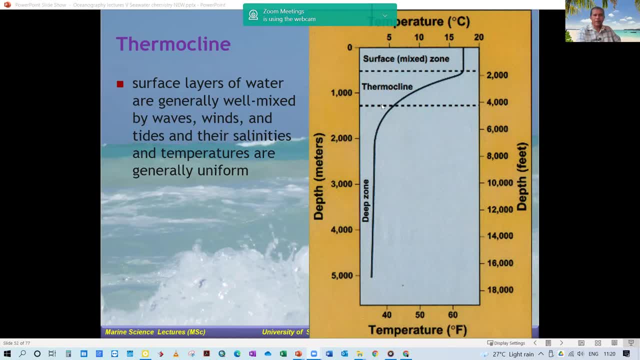 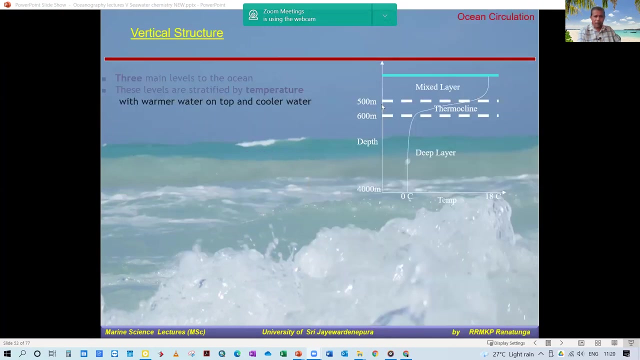 productive compared to the, the temperate country. because of this, because our waters are not really very productive, we think the other way, right, okay, so this is very important. this thermocline is a barrier for the organisms and similarly, you see, um, the same thing actually, the, the different layers, the mixed surface layer. 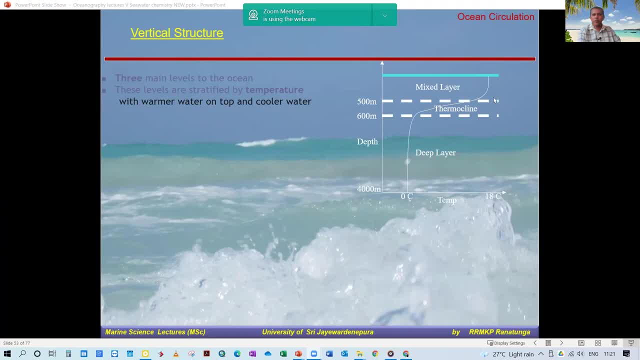 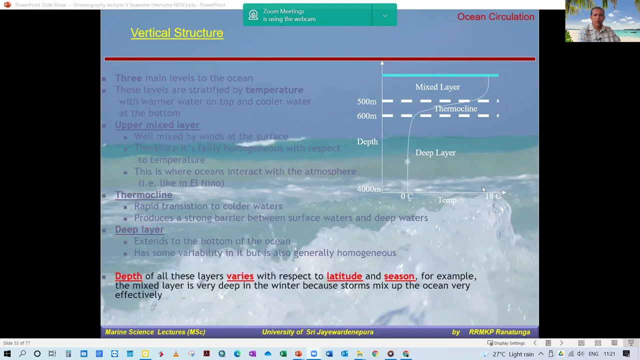 the deep layer. we call the three doc, three box model. i mean box to knock out the box. so that's, that's the typical, the vertical structure. that's the typical, the vertical structure, that's the typical, the vertical structure. so so that's where we have the, the thermal client and that very um. 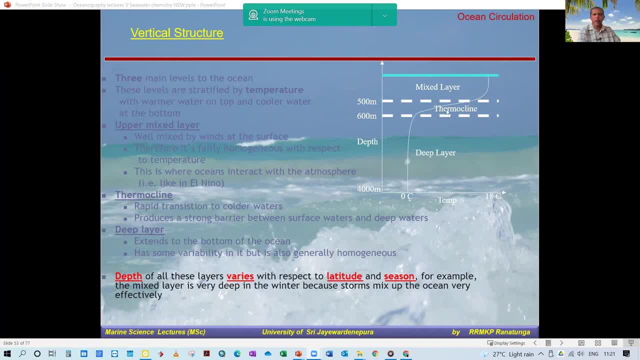 badly affect the marine organisms as well as productivity. but this- the thermocline deaths- change with the season, the time and many different aspects, but if you look at the temperature curve anywhere in the ocean, you will see something similar, especially if there is a. 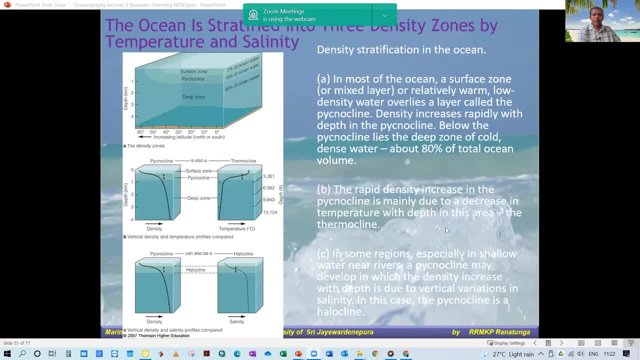 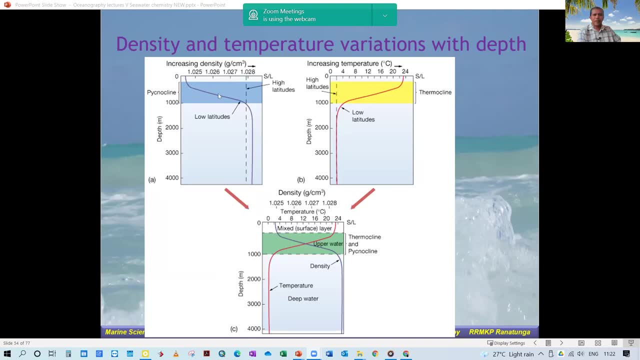 deep water in the tropical ocean side. so that's how it would look like And in these graphs you will see how the density change with the depth. and this is how the temperature change with the depth. And even if you look at the salinity, it will follow the same as the density, because 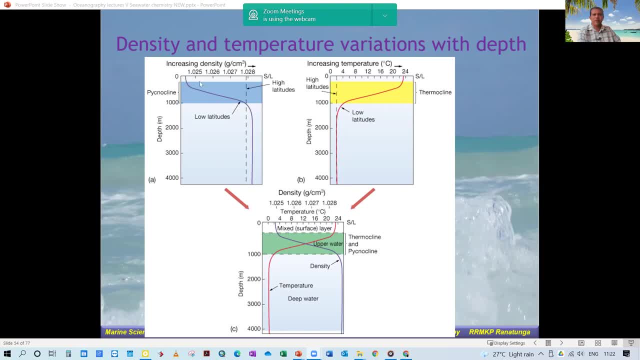 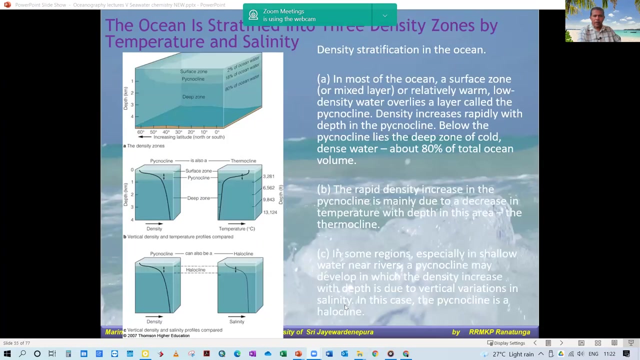 they are proportional to each other- the salinity versus the density- And this is affecting opposite direction, the temperature versus density. As you know, temperature and the density have opposite relations, and this is obvious in this graph as well, So that is something to look at. 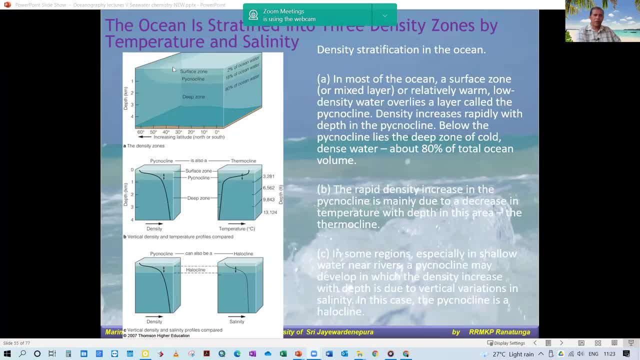 So you can see this three box model here: the surface zone, the middle zone and the deep zone. These boxes are like that. So here you see the pycnocline versus thermocline. Pycnocline is the density curve same as 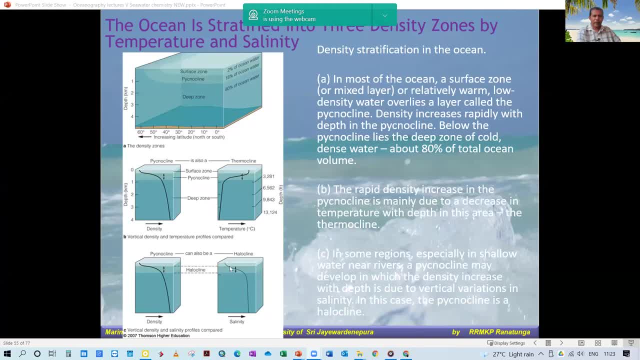 the salinity curve. You see, the halocline or the salinity curve is like this and the density curve is all right. so this is just to give you an idea how these physical parameters change with the ocean depths. This is badly affect the marine organisms as well as their products. 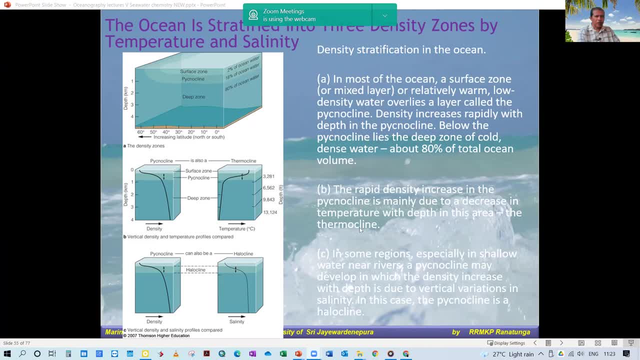 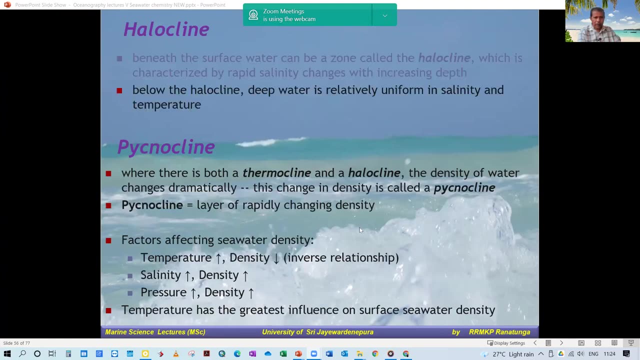 productivity. If you don't understand this one, try your best to understand. I mean, there's no something rocket science here. But if you have any question you can raise this right. So again, we are talking about this: clients, the hollow coin, halo coin and the salinity. 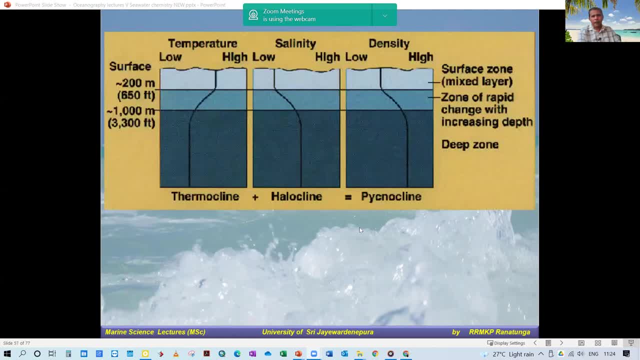 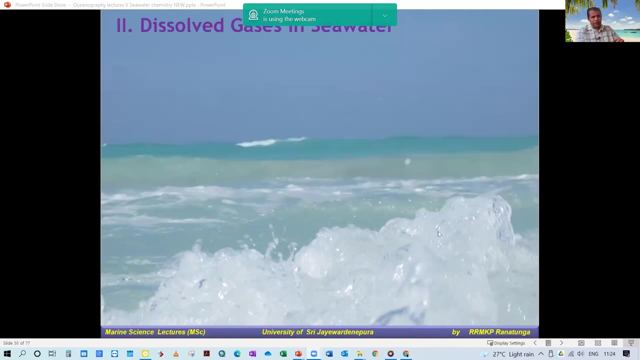 changes, the picno kind of the density changes, And we'll see how we put all these together. This is how it would look like the temperature curve, the salinity curves, density curves, when I put in a same scale right, Hope you got some idea from that And other than that. 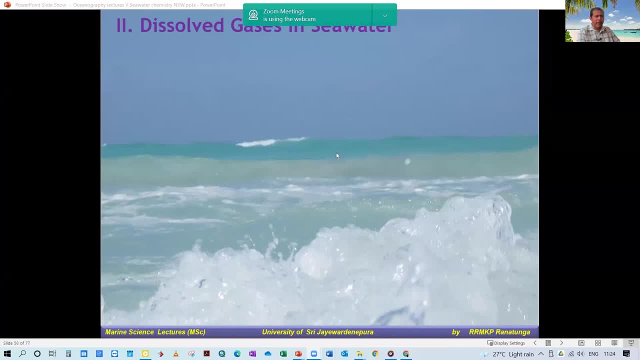 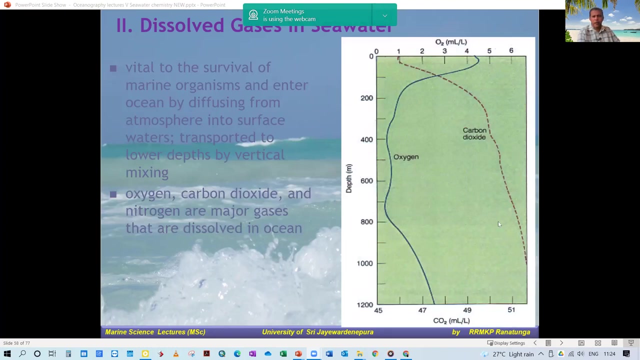 if you very briefly go through the different gases, how we change with the depth, especially the oxygen, carbon dioxide and nitrogen, how these change with the ocean depth, something very interesting to look at. And here you see the carbon dioxide curve in the dotted red color, at least in the dotted line, whereas the the solid line. 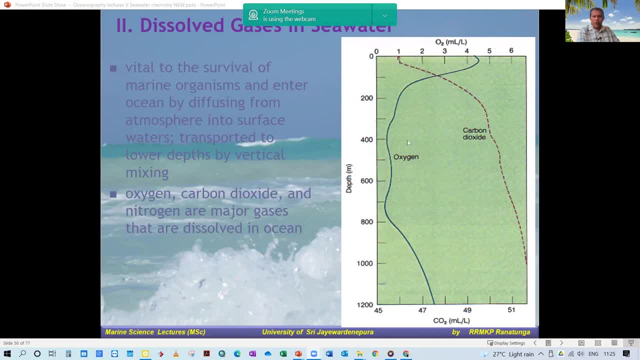 is the oxygen, As you can see that, the oxygen versus the carbon dioxide. those will look like something opposite, right, Opposite, proportional sort of a relationship, right? Can anyone think of why this opposite curve that we have for the carbon dioxide and oxygen? If you look? 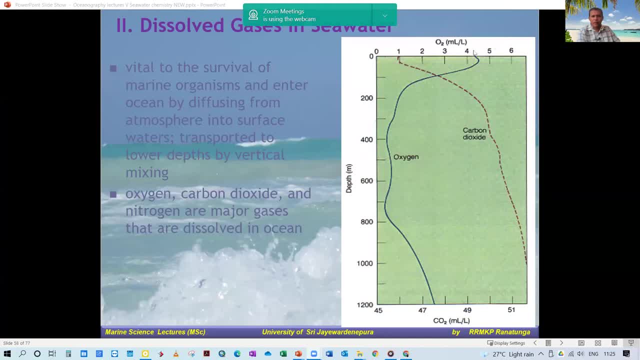 at the oxygen. I see the oxygen is higher in the surface waters but the getting very low in the deep waters. but in between you have a grow, a climb, oxygen climb. Now the oxygen climb here, but again in the very deep waters. 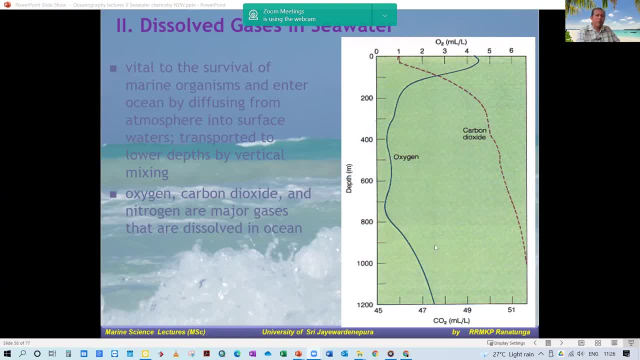 you see the oxygen increase again. So that is a typical curve you would experience for for the oxygen, Very unique. Can anyone think of why the oxygen is higher in the surface layers and why it is low in the bottom layers? Plants release oxygen by photosynthesis. Exactly, Very good. 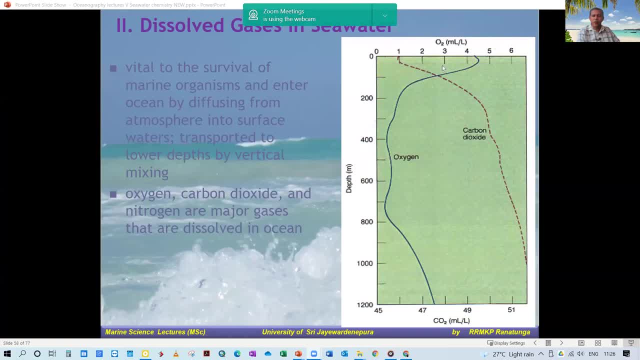 Right, That's very good thinking. because it's oxygen is produced by the plants, particularly the algae, Or particularly the plankton, where they are the primary producers, They have to release oxygen. and because there is not many phytoplankton in the bottom layers and 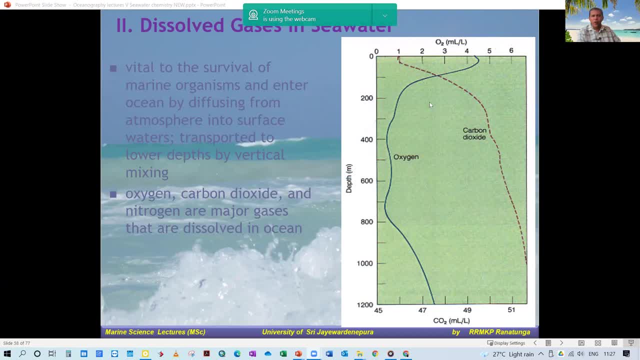 the production of oxygen is very low. Now the other thing is how much oxygen is dissolved in the water, because the oxygen dissolves easily in water When the turbulence is high. when there is a mix in the well, the oxygen dissolves very well. That's why you use 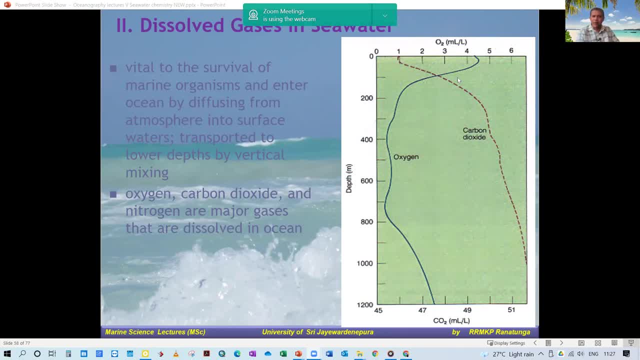 an aerator in your fish tank. So you have an Aerator and a pump. Another way is to make an Oxygen pump Right. it is not an oxygen pump Right, It's just an 팔 pump, where it pumps only the air. 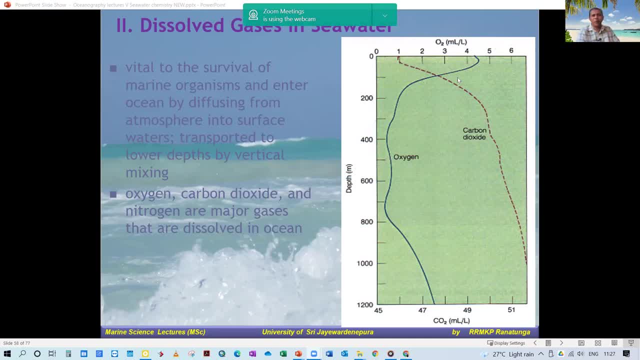 Now it's just a pump with air. pump air, the normal air, into the water. because of the turbulence that it creates. the oxygen dissolve easily with the turbulence. right wherever the turbulence is high, the oxygen dissolve easily. that's where you get higher oxygen in the surface layers, whereas the the lower and then and 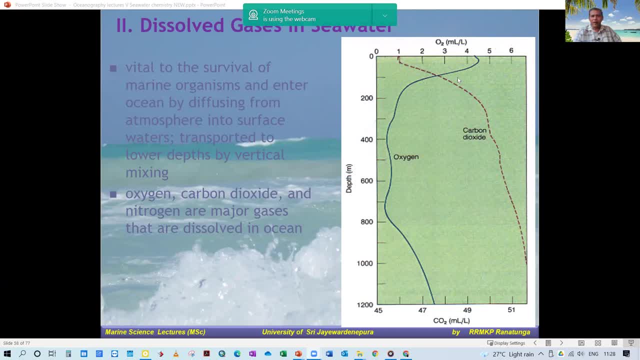 turbulence is very low in the bottom layers right. so the oxygen production is low and as well as the turbulence is very low, the both due to both reasons. so the oxygen is low. now there is another issue, because after, after certain depths, again the oxygen increases and that is because the oxygen dissolve easily with. 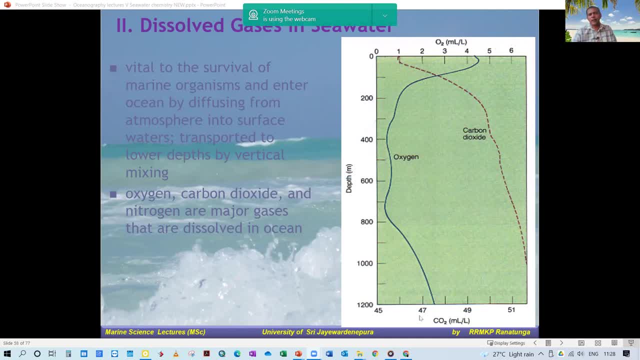 low temperatures or, on the other side, the oxygen retention power of the the water body decrease with increasing temperature. right when the higher temperatures the that water body cannot hold a lot of oxygen, that oxygen will release to the atmosphere. another thing that we need to remember is that the most of the 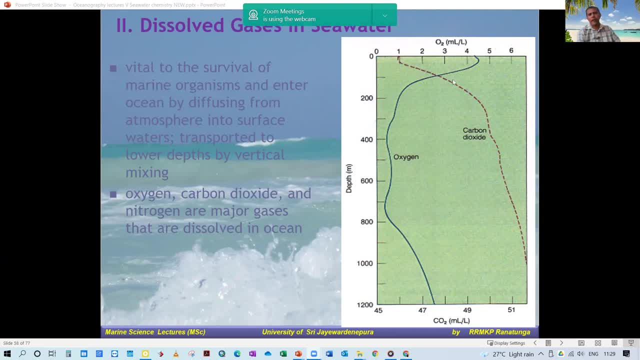 oxygen that produced in the, in this layers. since this oxygen they cannot be dissolved easily because, right, the, i mean not all oxygen will be dissolved here, and much of the oxygen that produced here they will release to the atmosphere. that's where the, the atmosphere, gets oxygen from, right. so 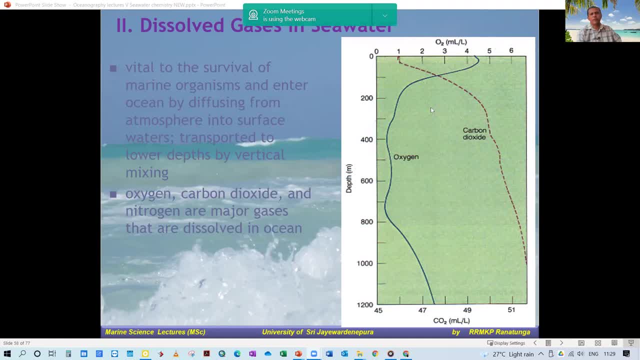 keep in mind that the very first thing, we took more than 50 percent of the, the oxygen in the atmosphere coming from the sea. that that's how we get the oxygen right. uh, so that's the oxygen curve. now the the other one is the carbon dioxide curve. 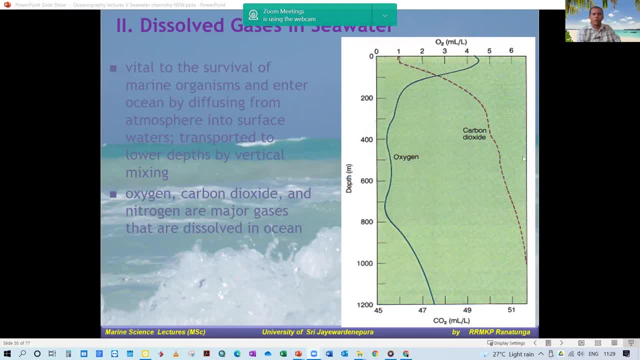 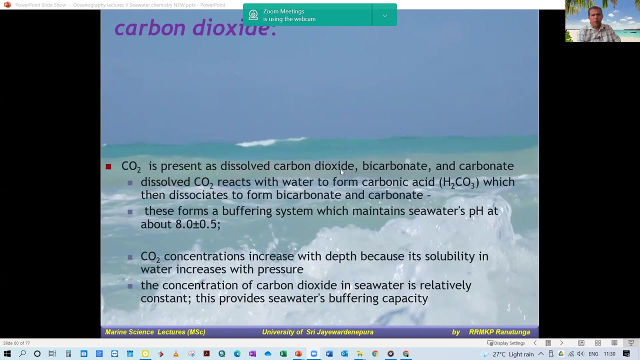 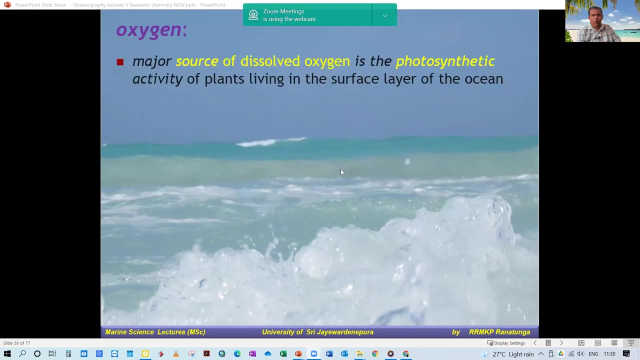 so it has the opposite, uh, sort of a representation here. so why the carbon dioxide is low in the surface layers? can anyone think of why the carbon dioxide low in in the surface layer? so we already talked about the oxygen, about the carbon dioxide, right, right, why the carbon dioxide is like this. 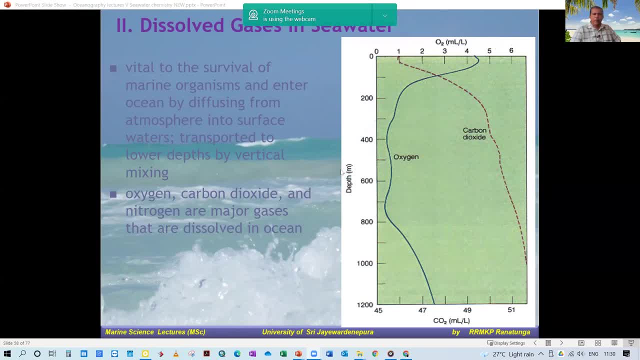 right, the carbon dioxide solubility. actually nothing to do with the turbulence or the mixing. the main reason for carbon dioxide dissolving power is with the pressure right. so imagine your the, the soft drinks, yeah, 있는 more we know. and that's where the carbon dioxide dissolves easily: in the bottom waters because of the high 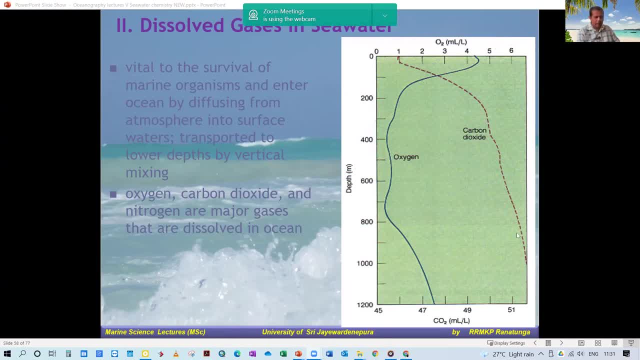 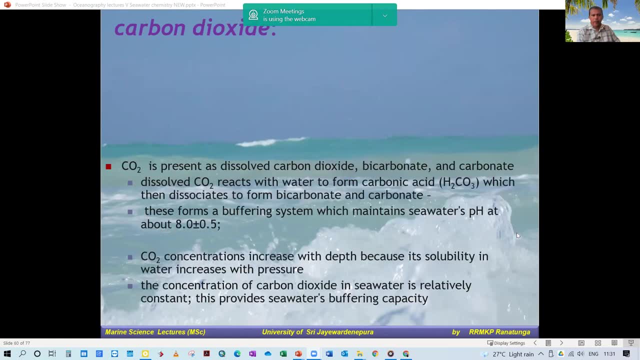 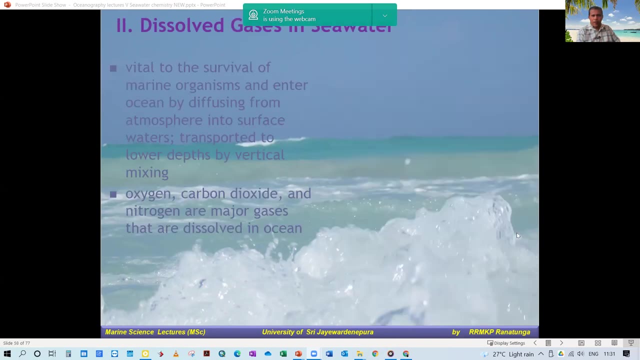 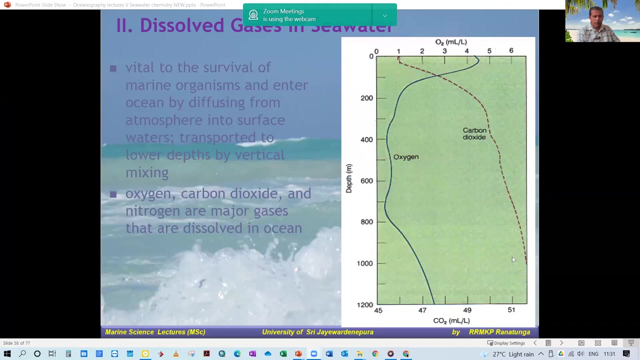 pressure, right. so it's completely different concept here. the carbon dioxide easily dissolves in the the deep waters when the pressure is very high, right. On the other hand, you see the in the bottom. after certain depth there's no huge change in the carbon dioxide because the, the solubility, doesn't change very much after that, right. 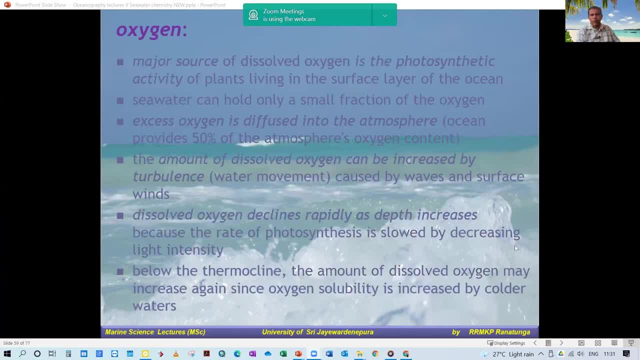 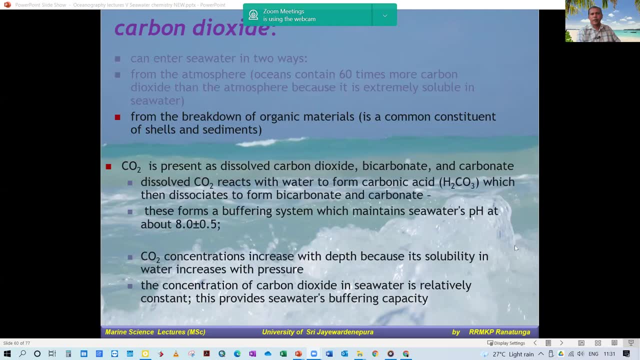 it's very much a constant, mainly because the the there is something called buffering activity. you know, the carbon dioxide dissolve in the water And at the same time, sometimes the it will produce carbonic acid, but on the other hand, the carbonic acid will break into the carbonate and the hydrogen ions. 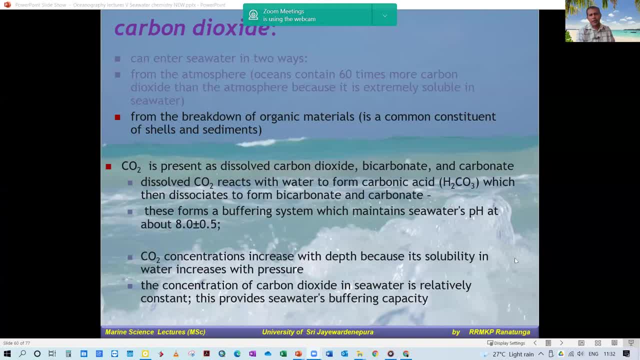 And the transition between the carbonic acid and the carbonate ions will keep the, the salinity, pretty much so the, the concentrations are- actually the pH in the water- relatively constant, right. So that's very important in the in the in the marine environment, right. 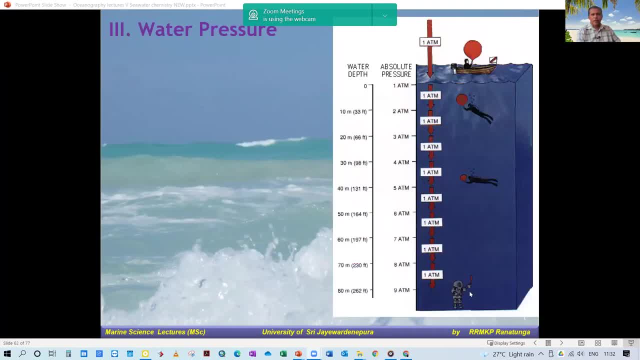 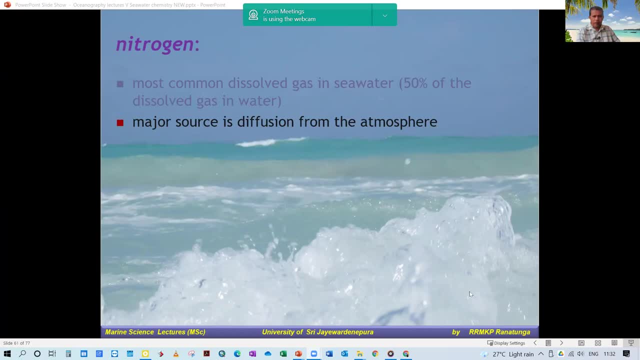 So the nitrogen doesn't so much. It has a huge influence. but the nitrogen, The ocean get the nitrogen from the very much, from the, the atmosphere, right, The nitrogen important for the marine organisms, for the, especially for the production of amino acid. but the nitrogen has something very important. 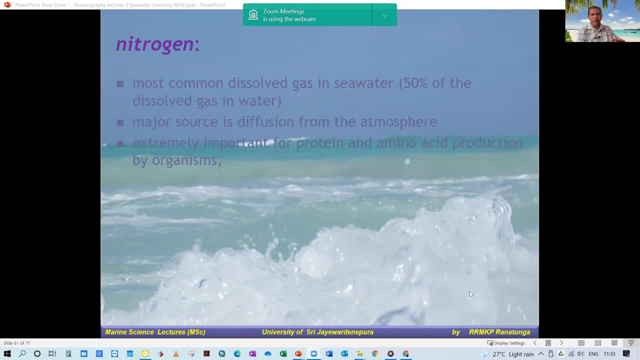 So who's going to be using it? Okay, Yes, Thank you. important for the some of the organism, for example human, especially if you are a diver right, this nitrogen going to cause a issue because the nitrogen solubility also increases with pressure right in the deeper water. if you deeper you go, there's more chances of dissolving nitrogen. 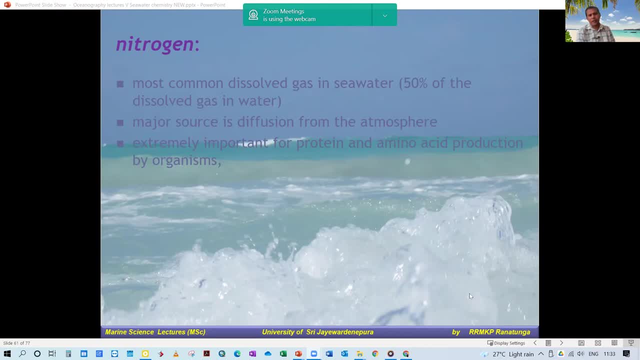 in your body. right. easily dissolve nitrogen in your body when in the deep waters, but if you come to surface at once, so then nitrogen start making bubbles right, like if that bubbles might block your blood vessels which can cause serious issues in divers right. so the nitrogen can be toxic. 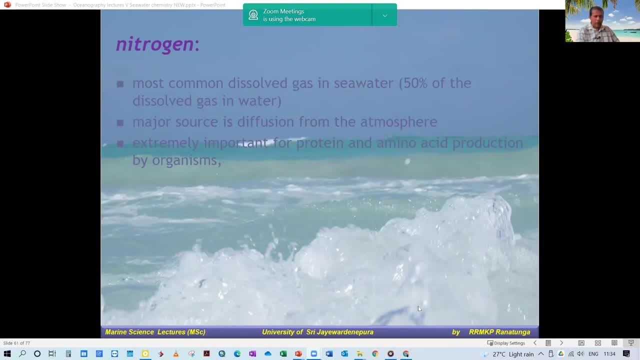 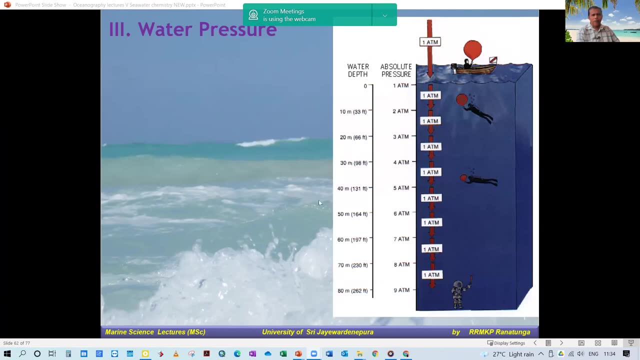 sometimes, and also it can cause some issues which called the bend all right, the, the other thing, the how the pressure change with the the ocean depths. this is very important. another phenomenon in the marine environment, as you can see in this uh sort of graph or infographics, if you carry a balloon like this, 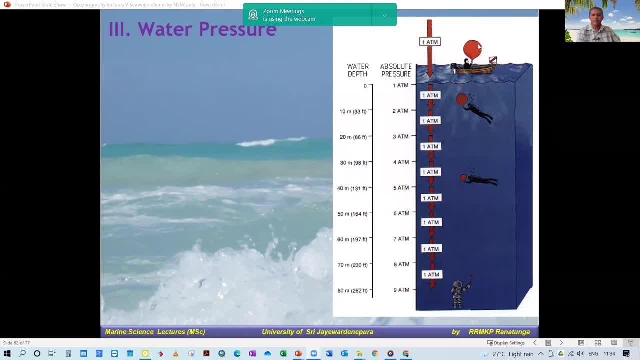 if you are a diver, you carry a balloon like this. you take it to the ocean bottoms and this is how it would look like with the bottom right. it can be very big at the surface and it will become smaller and smaller, which it shrinks because of the, the, the pressure right. every 10 meter you go deep, that will increase one atm. 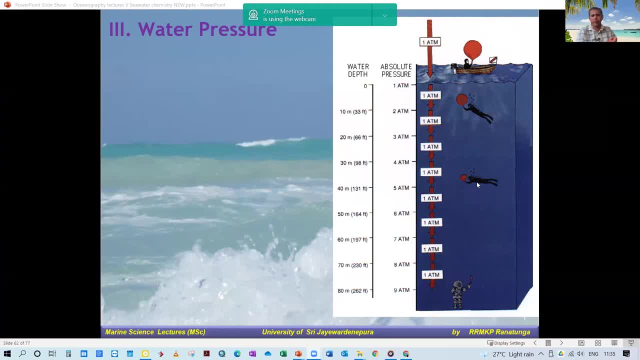 pressure, that will add on 180 m pressure, right so the in the sea surface and all the india in the coast or in the beach, you will have 180 m pressure, but next 10 meter in the water you will have another 180 m and and that will follow in every 10 meter, right? so if you go 30 meters, that means you. 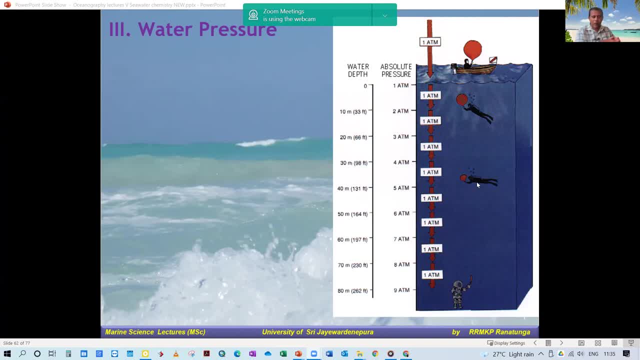 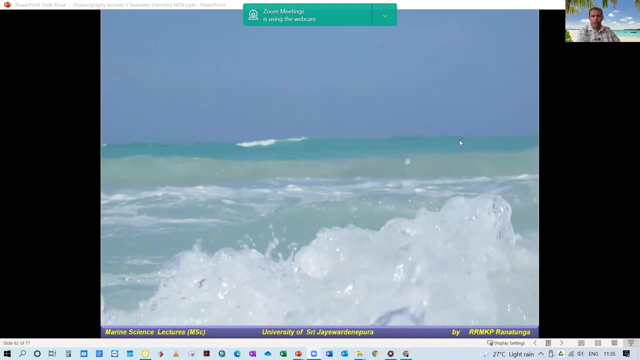 will have um 480 m actually, because there's already one in the atm and another three to be added. you will have 480 m pressure. so imagine in the deep waters how much pressure you can have all right, um. so that's the how the pressure um impact on you. now again how this affects the marine organisms, like 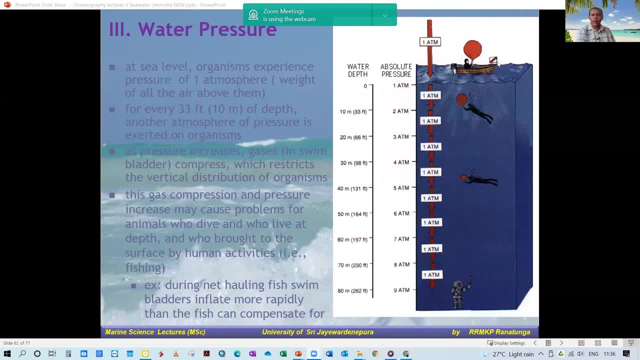 especially the, if the, the organism has a, have internal like uh spaces with the air or air sacks, now this is going to affect them the same as the balloon, if they have the air size, for example, if they have the lungs. luckily, fish, they don't have lungs, but they do have some some similar thing called the air sex. 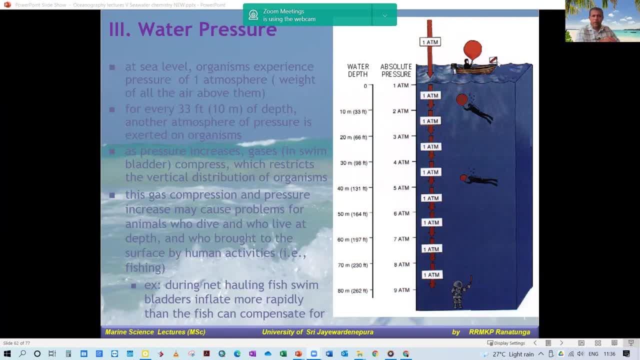 air bladder to keep the burns in the air. but that will affect the, the pressure will definitely for that right or even for the divers this is going to affect because their lungs- it's an air space- going to shrink as you go deep so you have less chance of breathing as you go deep because your lungs going to be smaller and 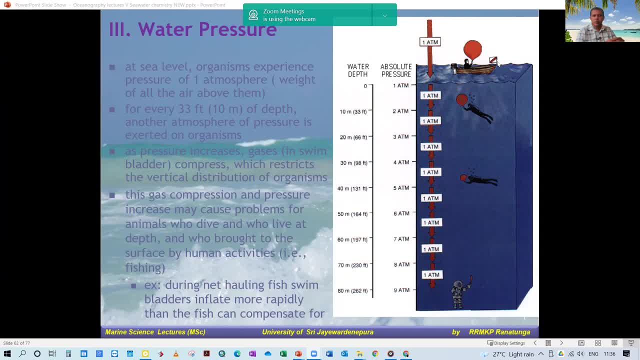 smaller and you have to the phase of the breathing have to increase as you go bottom, because that's lungs are very small. they can't hold a lot of oxygen right. so you have to be very careful in your in the deep waters, especially if you don't have like, if you're a free diver, hold in the breath for long period. 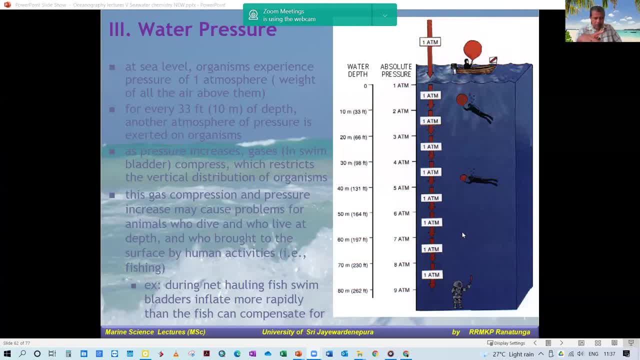 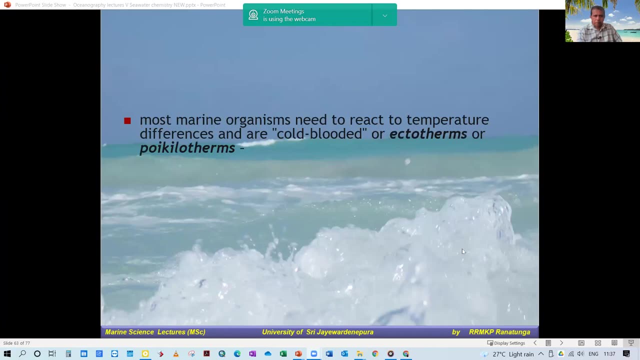 of time, if you go to bottom and then, with less oxygen and more carbon dioxide, you're going to loss your consciousness, right? so that can be an issue, right? okay, um, and that's where these- uh, most of the marine organisms has to be more like what we call the poikilotans. 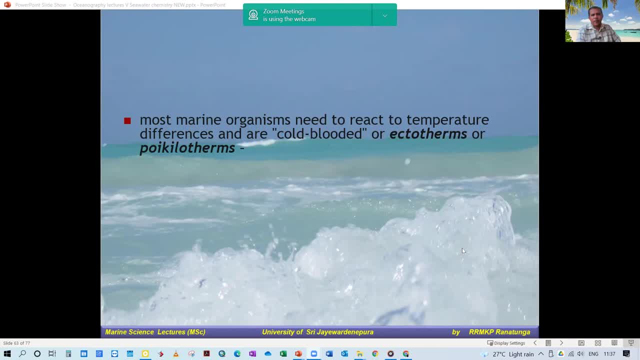 thermo conformers because the the water absorbed about temperature. if marine organisms or the aquatic organisms, they are water-based, they don't have to be thermo conformers. for the anaerobic and the aquatic organisms they are water-based. they are moreGPS-type organisms so they have to act with a 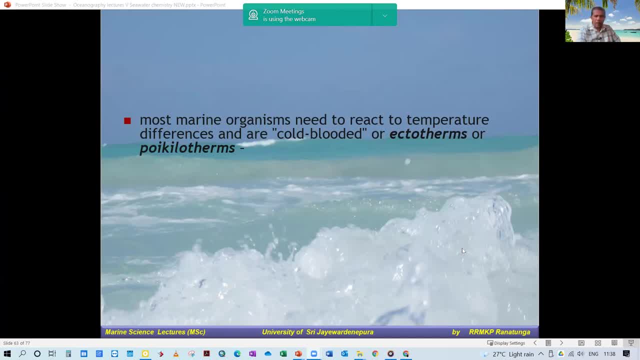 warm-blooded, they are going to lose their temperature a lot and that's where they become more osmo conformers or change their temperature with the environment. but this is different for marine mammals. they will have a lot of challenges to survive in the marine environment with this temperature, the salinity changes and the pressure as well, so they should have 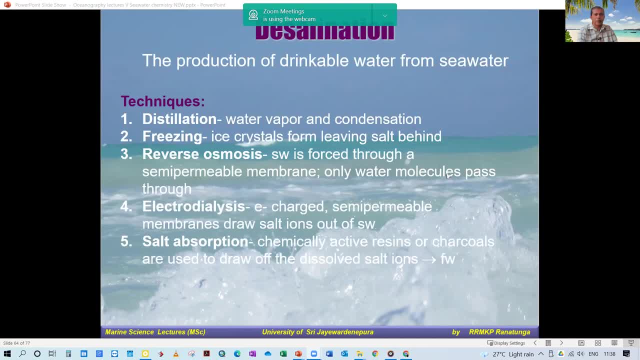 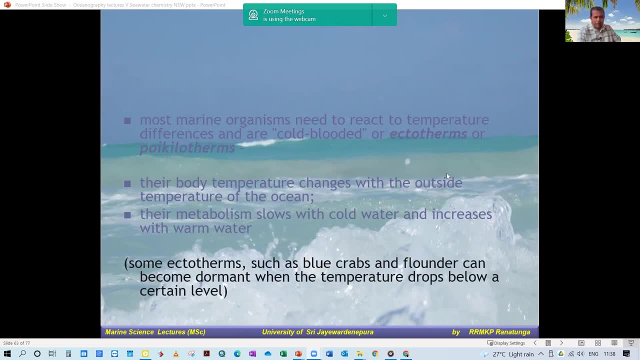 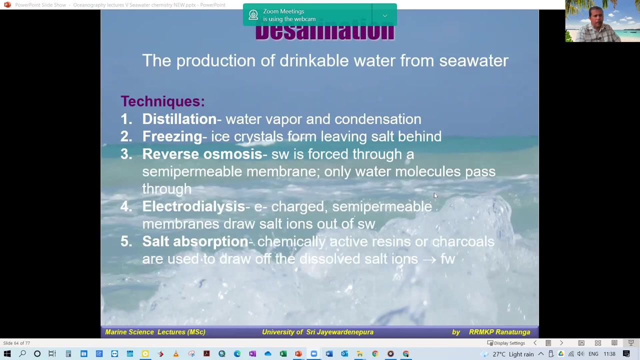 a lot of adaptation to this, right. so we'll look at these things in the, the when we talk about the marine ecological aspects, or maybe in your later years, right? okay, that's about the, the ocean chemistry a little bit, but on the other hand, we can know a little bit chemistry. 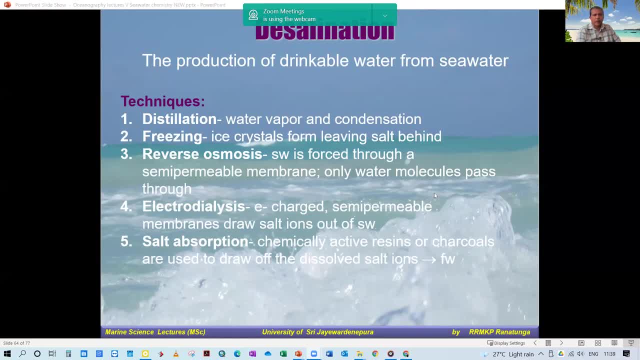 the ocean chemistry for many different purposes. for example, the like ocean acidity. if you want to measure the ocean acidity, you need to know the chemistry. on the other hand, we use the desalination, what you call the process called the desalination, where you remove the, the salinity, from the water and we can drink. 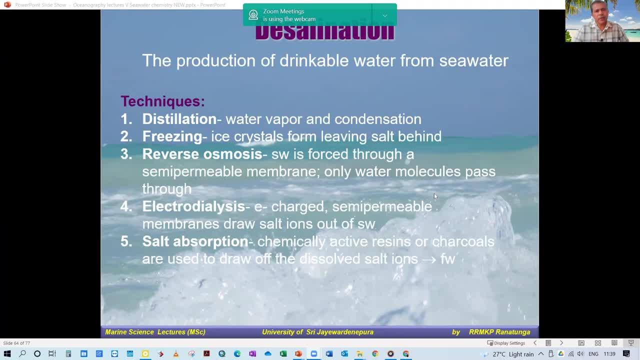 that water, especially in the areas where there is no enough water to drink, in the coastal areas. But if you have, If you have this sea around, you can use this desalination process to produce fresh water. now this has- this has been like- become more popular in the world, especially in the middle. 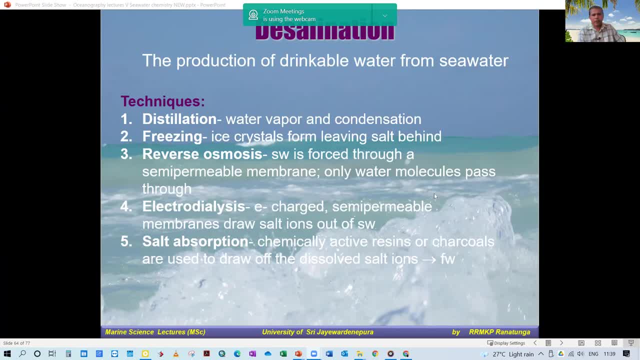 east countries they use, they take these techniques to get fresh water from the sea. now, even in Sri Lanka, in the remote areas in the coastal zone, when there is no the, the water supply from the sea. So if you are using the desalination process to get fresh water from the, the, the, the main. 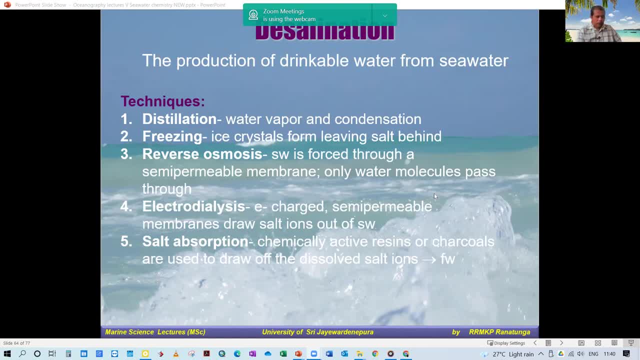 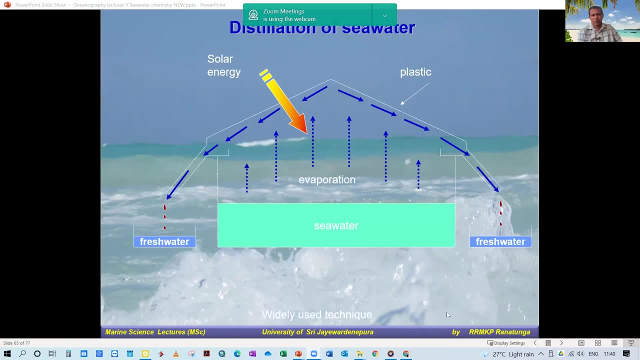 water supply boat, then they will go for this kind of a desalination and there are many different processes. I don't want to go into this. this just to, for your information, the sea water desalination process, either by um, um, uh, evaporation, right evaporation process. 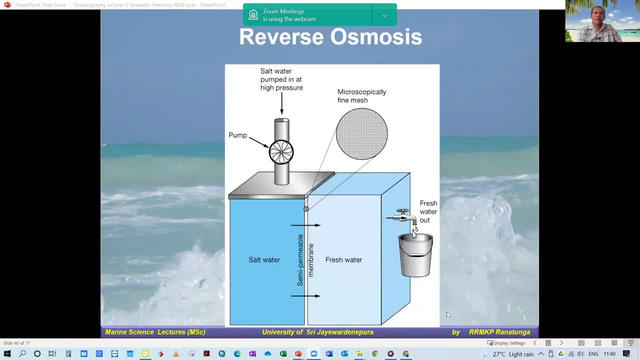 or else, uh, So this is the thing. So the sea water desalination, another process we call the reverse osmosis, we call the RO RO system, RO water filters, semi-permeable membrane- very important- even the pesticide and lot of pollutants will will be remain in the in this case. 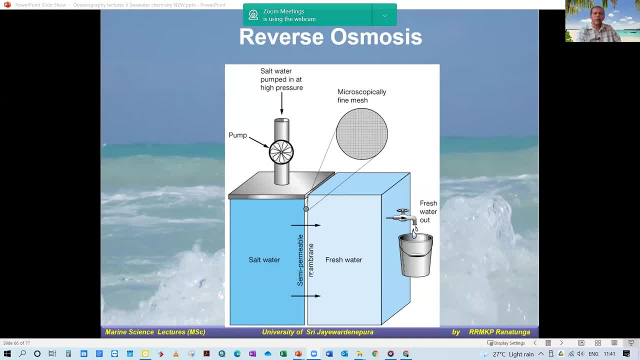 only the fresh water will press through the membrane, not even the essential minerals, right. but that's why in the, the water filters, they have to add the minerals. again, if you want to make it a drinking or drinking water, you have to add minerals artificially for RO waters, right. so keep in mind, especially if you are in the some areas, if you use 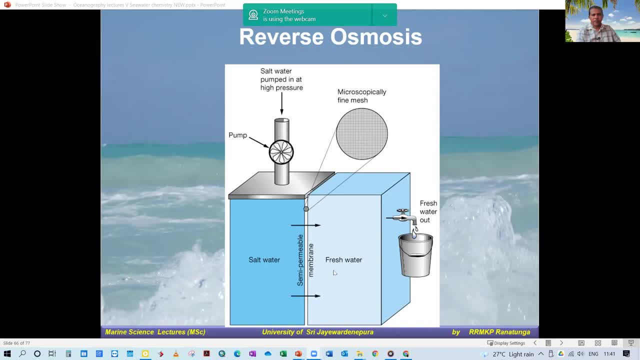 RO filters. make sure that you use proper filter systems, not only the filters を流入して. You don't want to be drinking or have a drinking water, so indeed, in the area for its safe to drinking water is, of course, can be released, but you do not use want to. 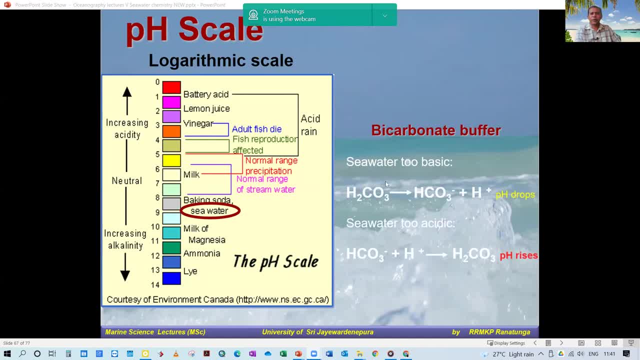 during this time that you can't use radical filters. you can also use Bол Joints at low pressure, a little low pressure, but you have to add a mineral cartridge, otherwise you will lose the essential minerals in the water. right, so that also important. okay, as I mentioned before the sea water, there is a buffering action. 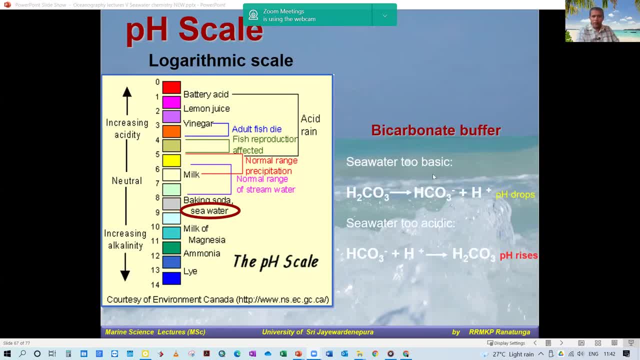 important. that's how it keeps the pH nearly constant. but since we are putting a lot of chemicals, especially the carbon dioxide, more, pump more into the sea and then the ocean keep the balance. the ocean lose the balance because we are putting too much carbon dioxide that the ocean 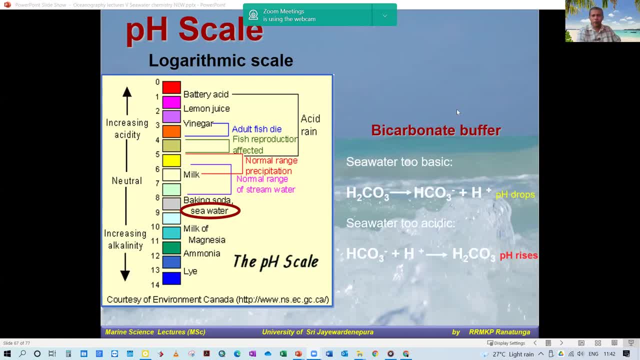 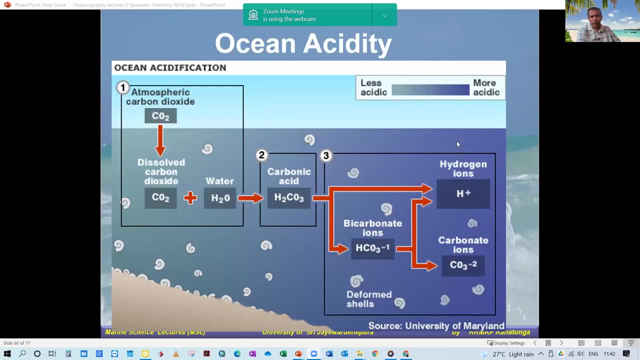 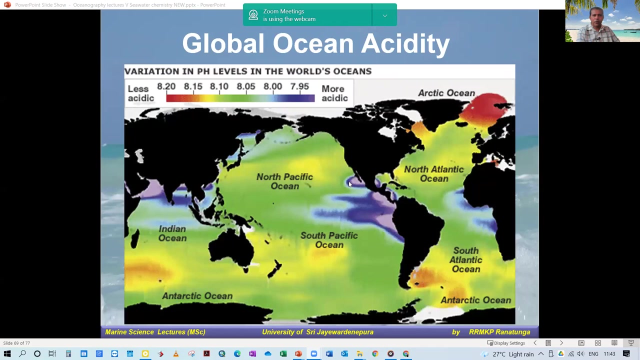 cannot withstand this buffering action. that's where they start raising the pH, what we call the ocean acidification. we will talk about this a little bit towards the end. how this form, this ocean acidity, ocean acidifications. toward the end, right. usually it has a relatively constant pH values which can change over time. 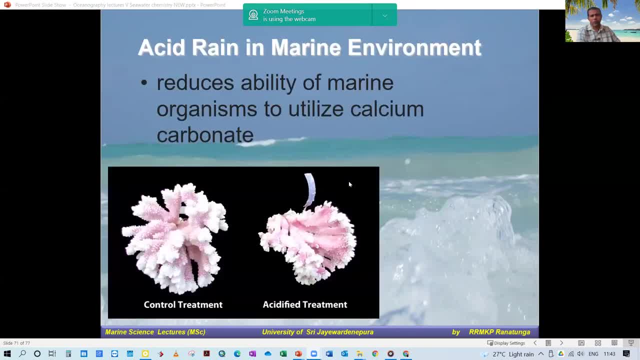 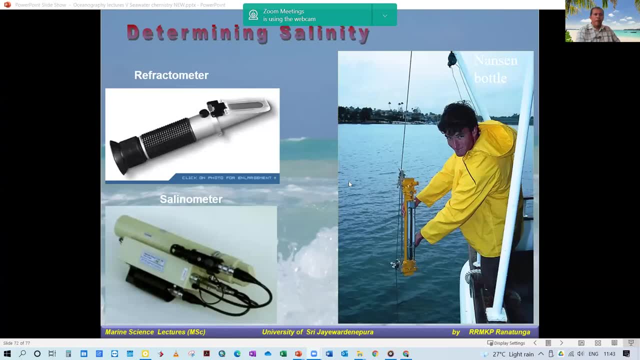 and these changes in ocean acidity going to affect a lot of organisms, which will especially be coral reefs- and we will discuss these things towards the end- and there are lots of instruments that can be used for detecting or measuring the ocean chemistry which we discussed in the very first practical session as well, like in this, the refractometer. 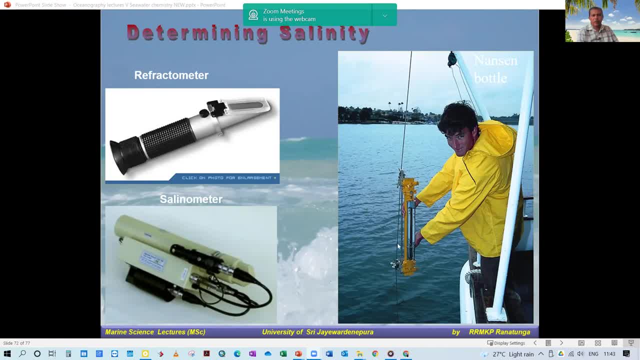 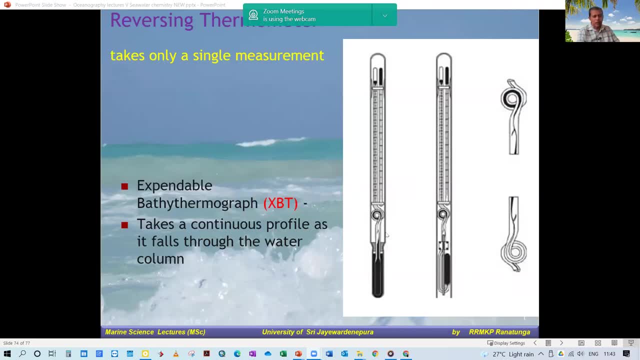 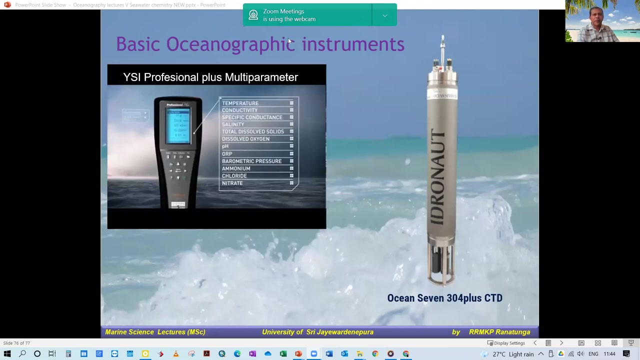 the selenometer and this kind of an ensign water samplers, and we will have another session on, like the oceanographic instrument, how they can be used, even this reversing thermometer. I think we will discuss previously the functions of this reversing thermometer and then, other than that, there are other instruments as well, something like a. 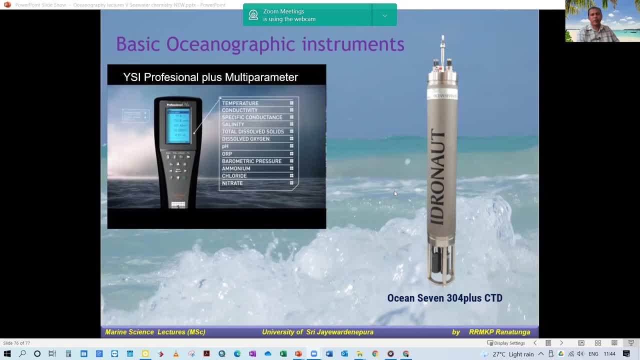 different electronic devices to measure the ocean chemistry, like this instrument we have already, like the ocean 730, it's a ctd, we call ctd, we call them as a data loggers, c. td means c means conductivity, t, temperature, d depth, with the depth it record. it records both.